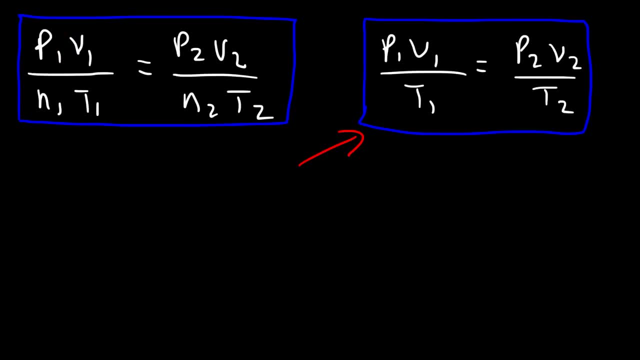 going to use this more often and I'm going to adjust it based on the problem. Now, if the moles is constant, I'm going to use this version, but I want you to be familiar with both of these equations. Another way in which you could derive the combined gas. 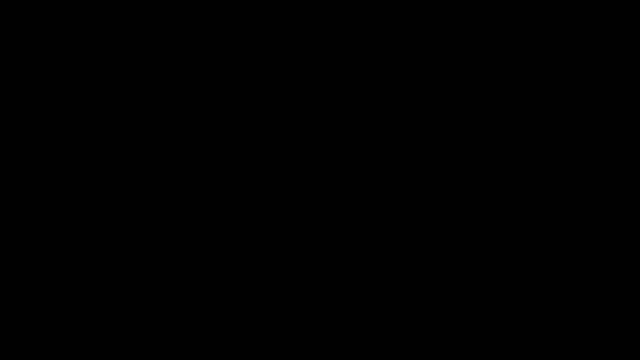 law is by combining the other gas laws. For example, we know that Boyle's law is P1- V1 is equal to P2, V2.. That's the equation that's associated with his law. And then we have Charles law, which is V1 over T1, that's equal to V2 over T2.. 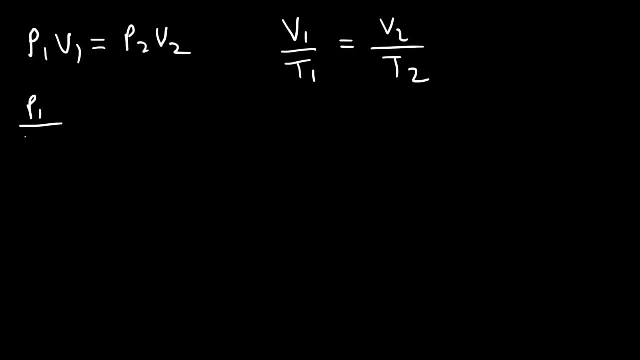 And then we have Gay-Lussac's law: P1 over T1 is equal to P2 over T2. and now have a Goddard's law: V1 over N1 is equal to V2 over N2.. So now let's combine these four equations into a single law. 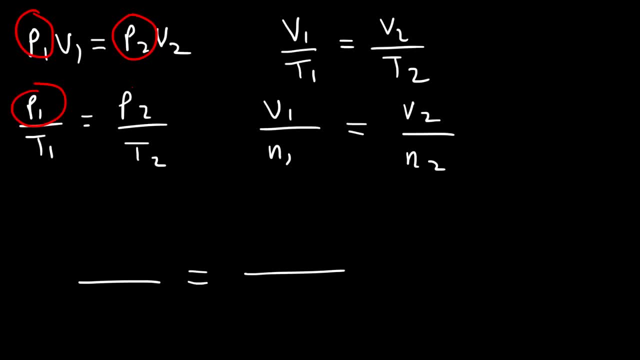 So notice that pressure is always in a numerator, so therefore I'm going to put it in a numerator of the equation below. So I'm going to put P1 on the left, P2 on the right. Now notice that volume is also on the top of the fraction, so I'm going to put that. 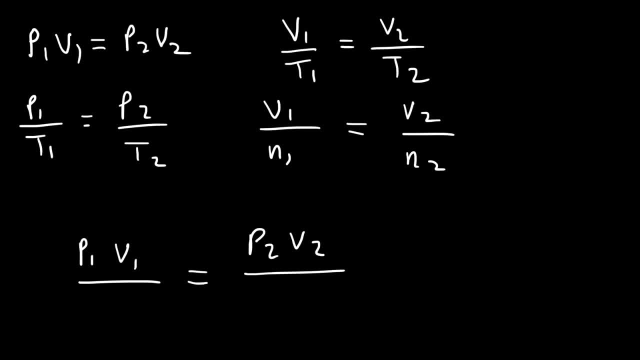 on top as well, So V1 and V2.. Next, temperature is always in a denominator, so I'm going to put that here: T1 and T2.. And notice that the moles is in the denominator as well, And so you get the same equation: the combined gas law. 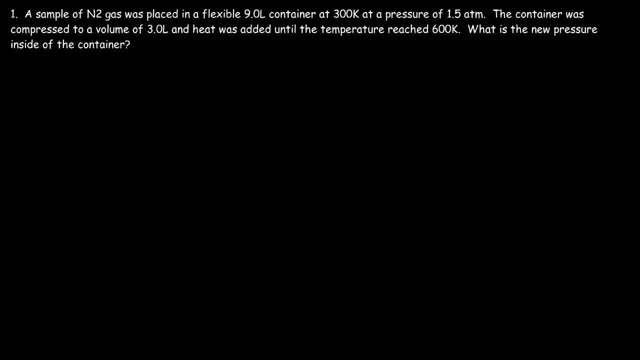 Now let's start with this problem. A sample of nitrogen gas was placed in a flexible 9 liter container at 300 Kelvin, at a pressure of 1.5 atm. The container was compressed to a volume of 3 liters and heat was added until the temperature. 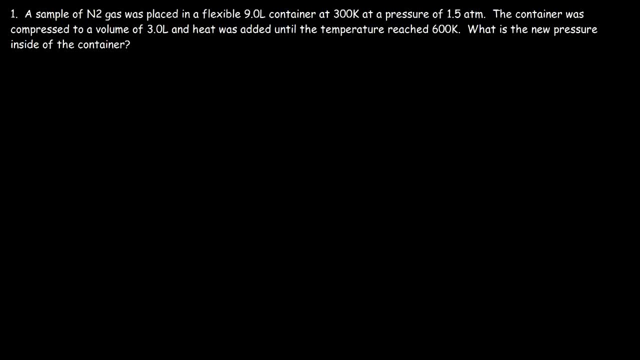 reached 600 Kelvin. What is the new pressure inside of the container? Now let's see if we can get the answer by looking at this conceptually. So the volume was decreased from 9 liters to 3 liters, So I'm going to put it was divided by 3.5. 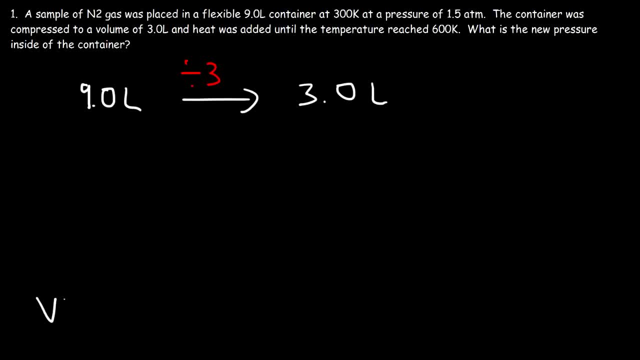 Now, if you decrease the volume according to Boyle's law, what's going to happen to the pressure? Now, according to Boyle's law, pressure and volume are inversely related. So if the volume goes down, the pressure is going to go up. 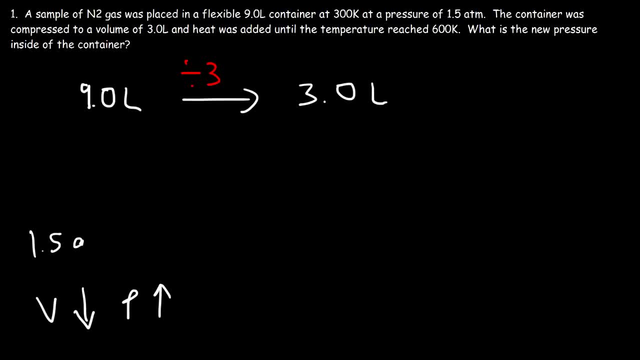 Now the pressure is currently 1.5 atm. So if we decrease it, if we decrease the volume by a factor of 3, the pressure should increase by a factor of 3.. 1.5 times 3 is 4.5.. 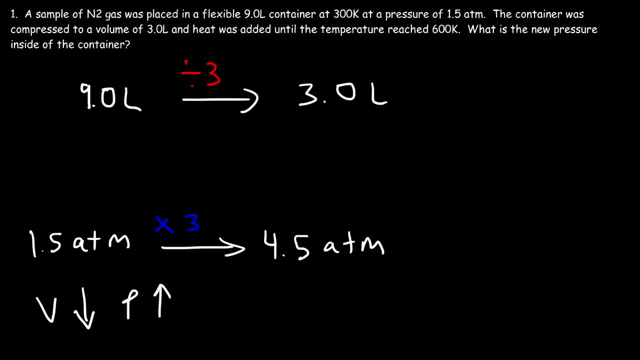 So that's what it should be. due to the effects of the change in volume alone, Now the temperature changes as well. Initially the temperature was 300 Kelvin. Now it increased to 600 Kelvin. So we multiply the temperature by a factor of 2.. 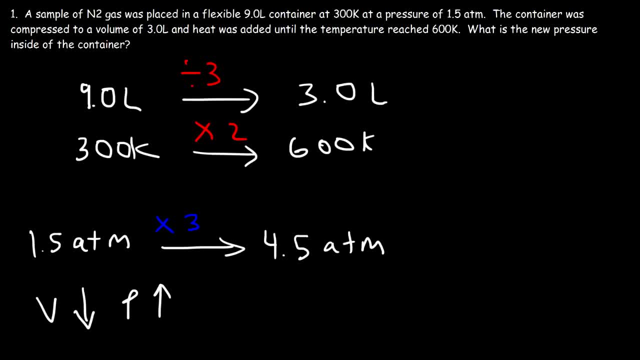 Now Gay-Lussac's law connects temperature and pressure together. Gay-Lussac's law states that 1.5 times 3 is 4.5.. 1.5 times 3 is 4.5.. 1.5 times 3 is 4.5.. 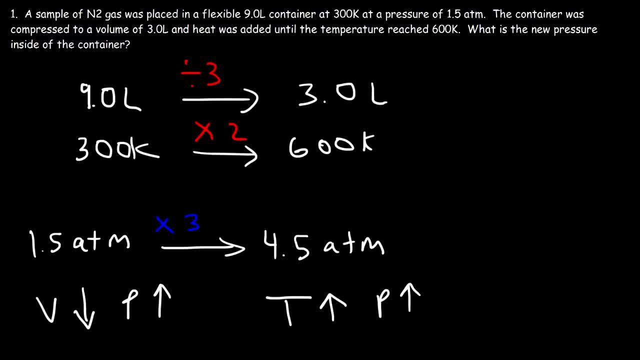 As the temperature goes up, the pressure will go up proportionally. So if the temperature goes up by a factor of 2, the pressure should also go up by a factor of 2.. So we're going to multiply this value by 2.. 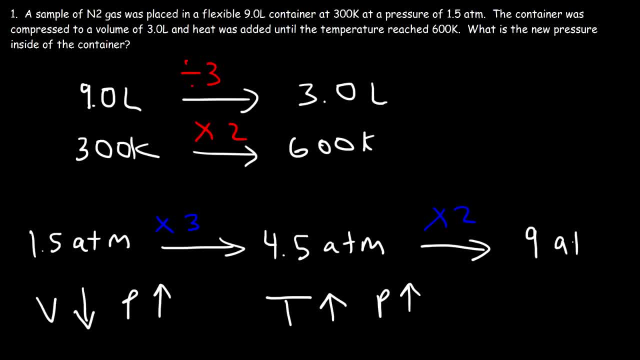 4.5 times 2 is 9.. So therefore, the new pressure should be 9 atm, And let's confirm that answer with the calculator. So let's write down what we know: V1, the original volume is 9 liters, T1 is 300 Kelvin and P1 is 1.5 atm. 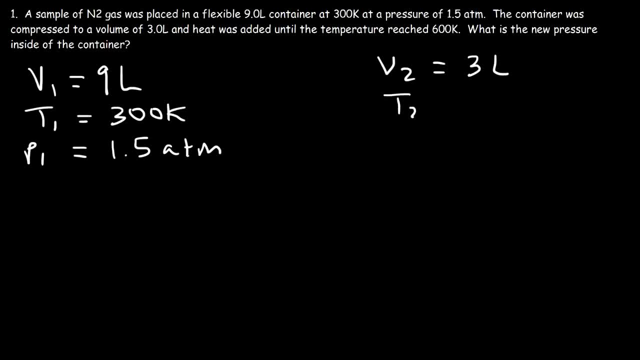 V2 is 3 liters, T2 is 600 Kelvin and P2 is what we're looking for. So that's what we've got to find. So that's what we've got to find. So let's start with this equation: P1, V1 over T1 is equal to P2. V2 divided by T2.. 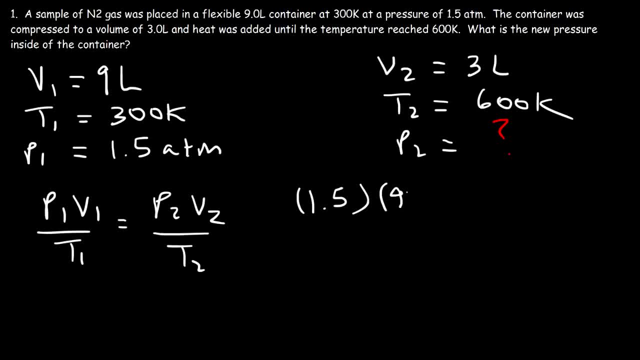 So P1 is 1.5,, V1 is 9, and T1 is 300.. P2, we're looking for that- T2 is, I mean, V2 is 3, and T2 is 600.. So let's cross multiply. 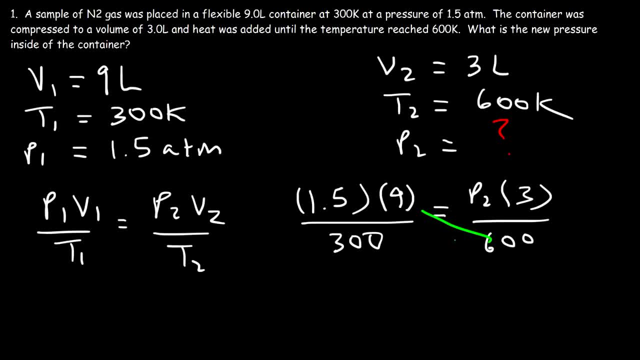 We're going to multiply 1.5 times 3.5.. We're going to multiply 1.5 times 3.5.. We're going to multiply 1.5 times 3.5.. So that's 9 times 600.. 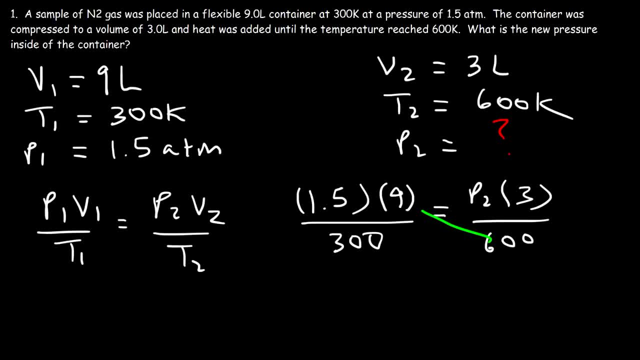 So that's 9 times 600.. 9 times 600.. And you should get 8,100.. Next we're going to multiply P2 by 303.. 300 times 3 is 900.. So that's 900 times P2.. 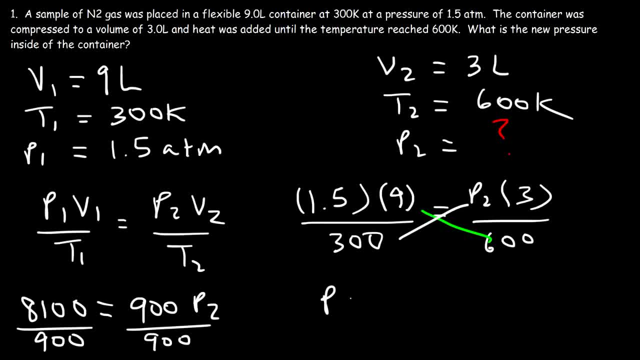 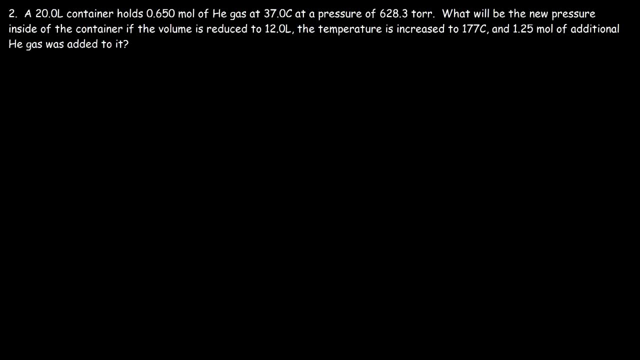 Now let's divide both sides by 900.. 8,100 divided by 900 is nine, And so you do get the same answer. And so you do get the same answer: 9 ATM. Let's work on this one. A 20 liter container holds 0.65 moles of helium gas. 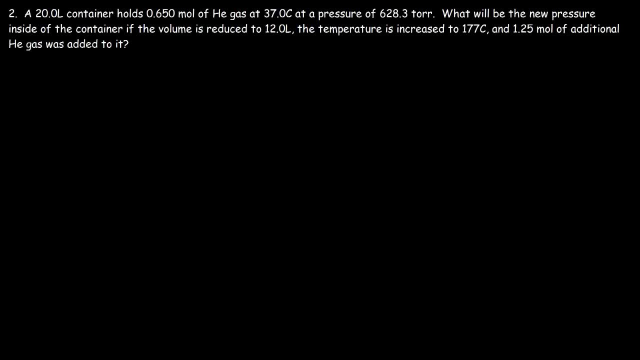 at 37 degrees Celsius at a pressure of 628.3 torr. What will be the new pressure inside of the container if the volume is reduced to 12 liters and if the temperature is increased to 177 Celsius and if 1.25 moles of additional? 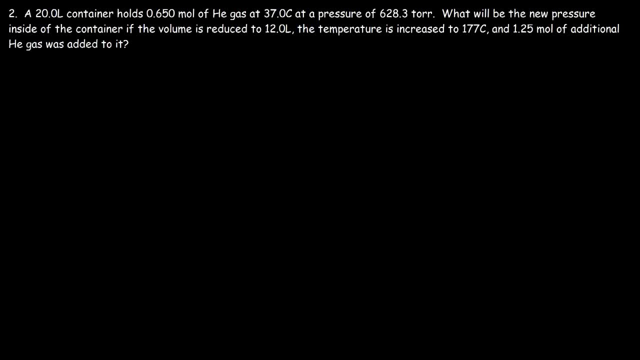 gas was added to it. Go ahead and try this problem. I'm going to make a list of what we have. So V1 is 20 liters. N1 is 0.65 moles. The temperature is 37 Celsius. Now, when using this formula, or basically almost any formulas associated with gas, 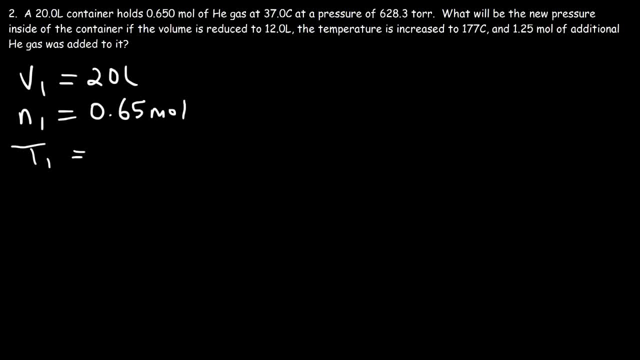 laws, the temperature has to be in Kelvin. The only time you can really use a Celsius temperature is if you see, like delta T in the equation. If you don't see it, if you see just T, always use the Kelvin temperature. The difference in 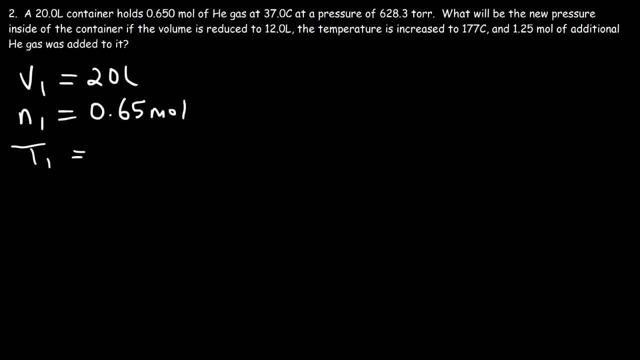 temperature, be it in Celsius or Kelvin, will be the same. But if you're multiplying or dividing by a temperature, then make sure you use the Kelvin unit, not the Celsius unit. So if you don't see a triangle next to the T, 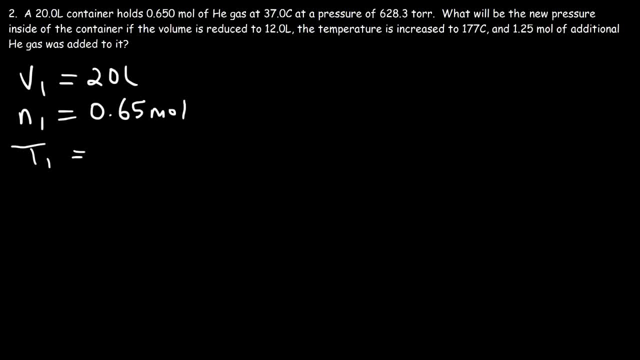 variable always use the Kelvin temperature, So we need to add 273 to 37., So that's going to be 310 Kelvin. P1 is 628.3 torr. Now we don't need to change this unit For this equation where you have P1 and P2,. 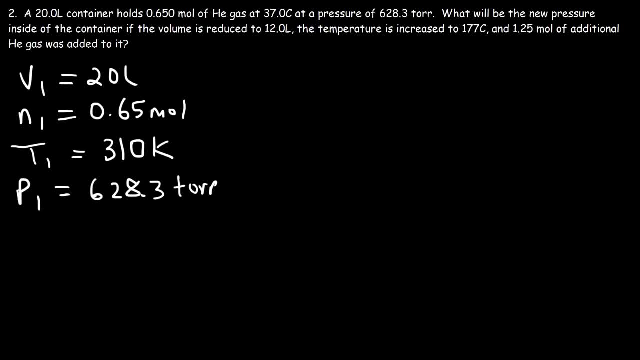 if P1 is in torr, then P2 is going to be in torr. If V1 is in milliliters, V2 should be in milliliters. Those units simply have to match. But the temperature has to be in Kelvin. If you put it in Celsius you will not get the 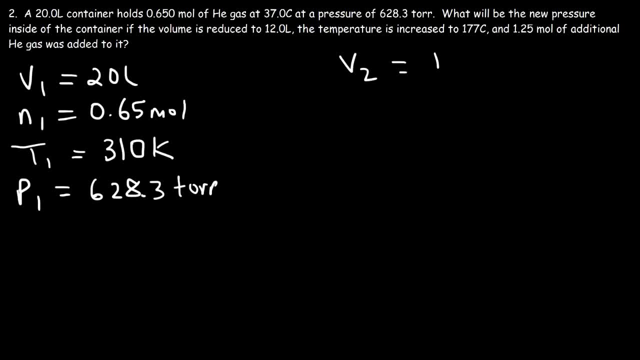 right answer. Now V2, it's 12 liters. What's N2 in this problem? Now, 1.25 moles of additional helium gas was added to it, So we got to add 0.65. Plus the additional 1.25. And so the final amount is 1.9 moles. Now T2, we need 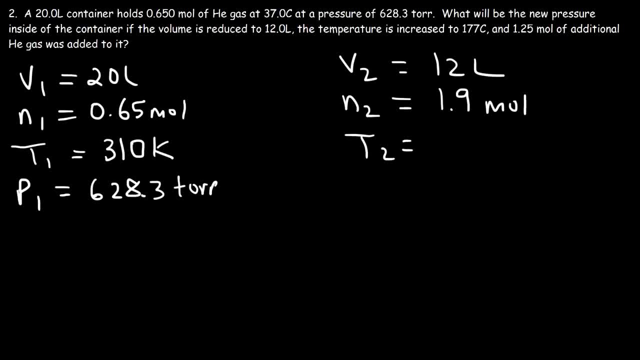 to convert the Celsius into Kelvin. So we're going to add 273 to 177, and that will give us a temperature of 450 Kelvin, And the last thing we need to do is calculate P2, which is going to be in torr. 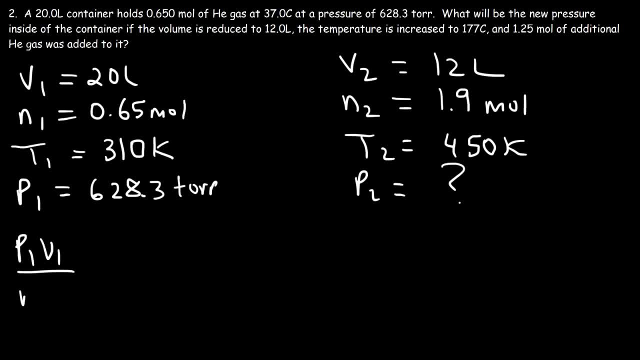 So let's use this equation: P1- V1 divided by N1- T1 is equal to P2- V2 over N2- T2.. So P1 is 628.3 torr, V1 is 20.. N1 is 0.65.. And T1 is 310.. That's equal to P2 times V2,. 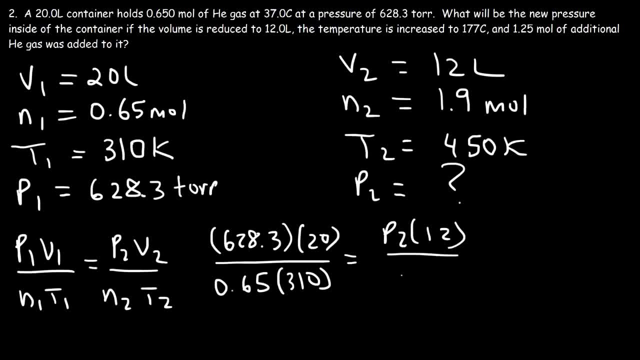 which is 12, divided by N2, T2.. Which is 1.9, times T2, and that's 450.. So now, at this point, all we need to do is just Math. so let's cross, multiply. So I'm going to multiply 628.3 by 20 and then